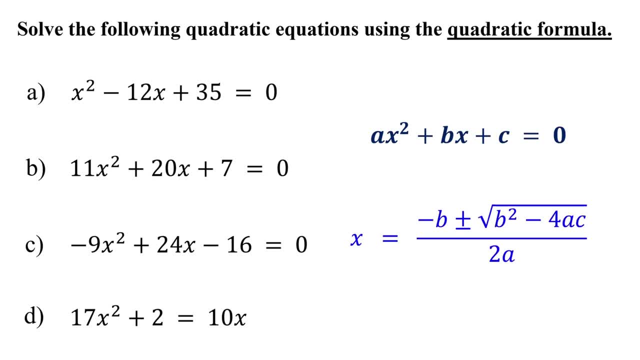 the quadratic formula is given by: x equals negative b plus or minus the square root of b squared minus 4ac, all over 2a. Here x represents the solutions and a, b and c are the coefficients of the quadratic equation. If a quadratic equation is given in standard form, 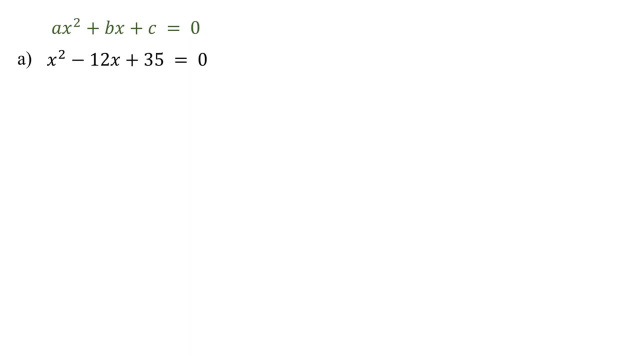 as in this example, our first step is to identify the values of the coefficients. Here the value of a is 1, b is negative 12, and c is 35. Next we write down the quadratic formula. Then we substitute the values of a, b and c into the formula. 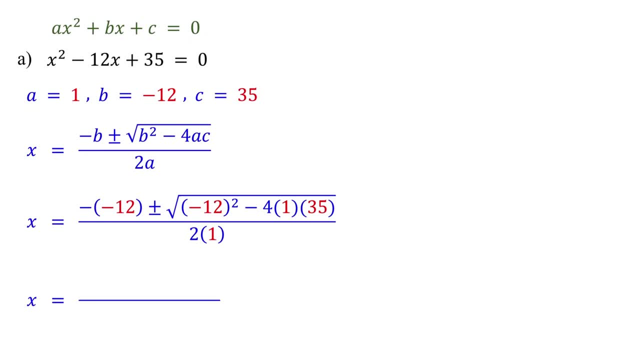 Now we simplify this: In the numerator the negative of negative 12 is positive 12, right Negative 12 squared is negative 12 times negative 12, which gives us 144.. 4 times 1 is 4, and 4 times 35 is 140.. In the denominator we have 2 times 1,, which equals 2.. 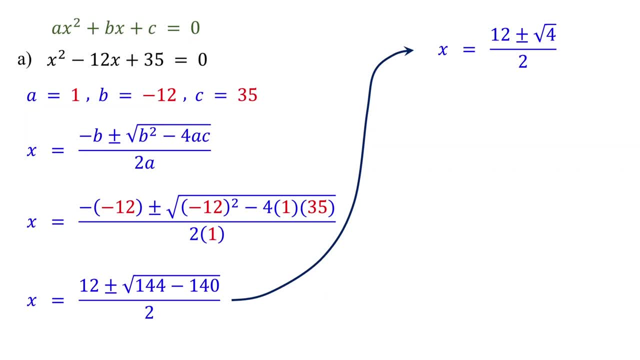 144 minus 140 is 4,. right, The square root of 4 is 2.. This is the same as x equals 12 plus 2 over 2, or x equals 12 minus 2 over 2.. 12 plus 2 is 14, and 12 minus 2 is 10.. 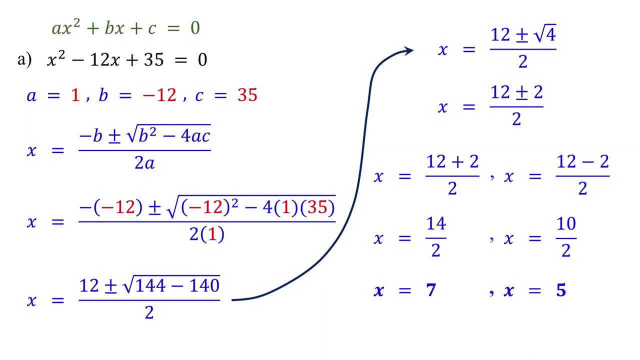 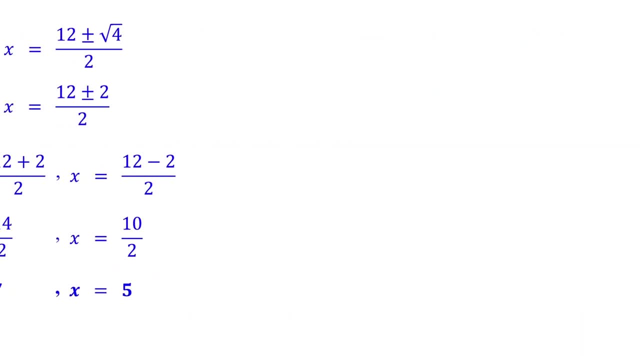 Dividing 14 by 2 gives us 7, and dividing 10 by 2 gives us 5.. Therefore, the solutions are x equals 7 or x equals 5.. by substituting them back into the original equation, Substituting 7,, 7 squared is 49, and 12 times 7 is 84.. 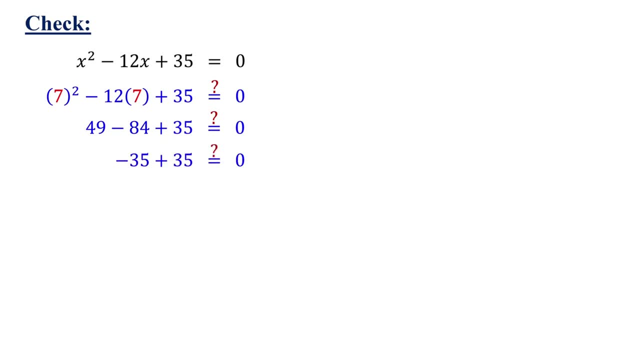 49 minus 84 is negative 35, and this equals 0, right. Similarly, substituting 5,, 5 squared is 25, and 12 times 5 is 60.. 25 minus 60 is negative 35, and this equals 0.. 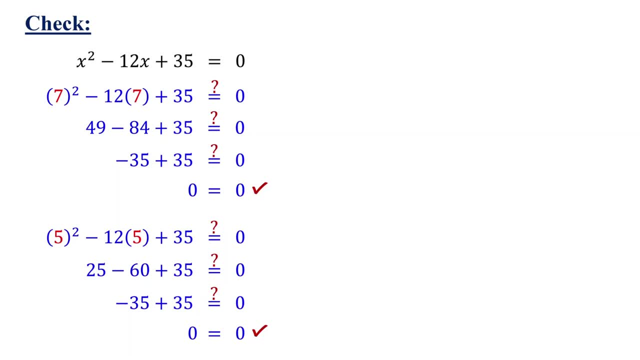 As you can see, both 7 and 5 are valid solutions. We can actually solve this quadratic equation more easily and quickly using the factoring method, as it is simple to find two numbers that multiply to give 35 and add up to negative 12.. 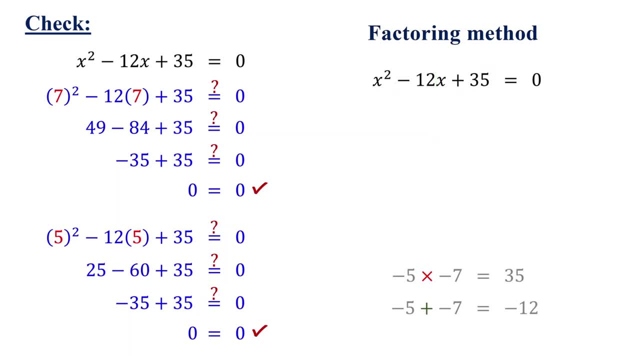 These numbers are negative 5 and negative 7, right? So when we factor this quadratic equation, it becomes x minus 5 times x minus 7, which equals 0.. Now, setting each factor equal to 0 and solving for x gives us the solutions. 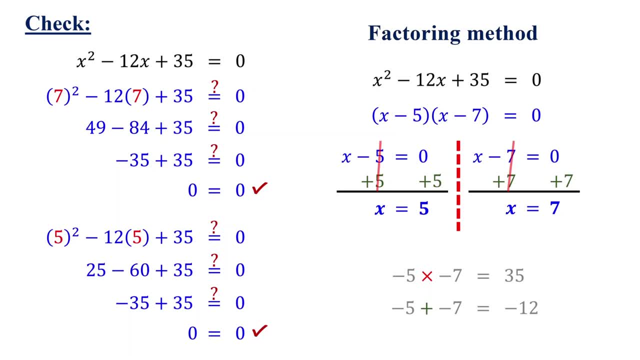 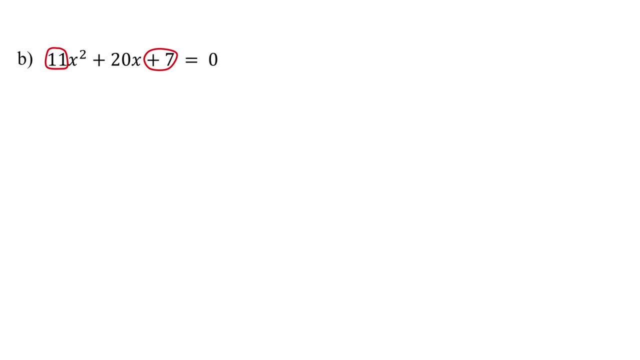 As you can see, the factoring method is easier and faster for this example right. However, not every quadratic equation can be factored, but all can be solved using the quadratic formula. For instance, in the next example, it is difficult to find two numbers that multiply to give the product of 11 and 7 and add up to 20.. 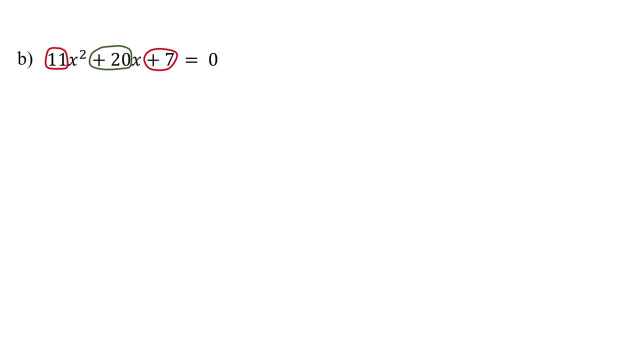 Can you find these numbers? It is challenging, right? Although it is hard to factor, we can easily solve it using the quadratic formula, Since it is in standard form. our first step is to identify the values of the coefficients: a is 11,, b is 20, and c is 7.. 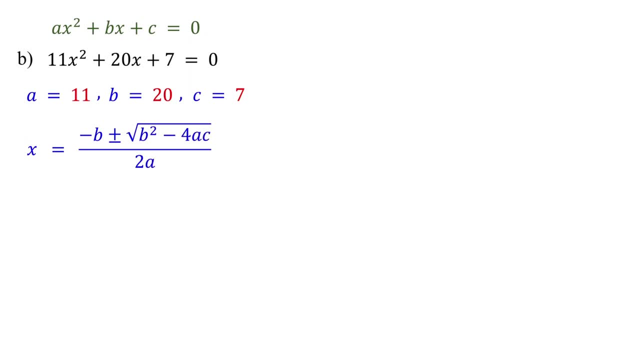 Next write down the quadratic formula. Then substitute the values of a, b and c into the formula. Now simplify this: Inside the square root, 20.. 20 squared is 400.. 4 times 11 is 44, and 44 times 7 is 308.. 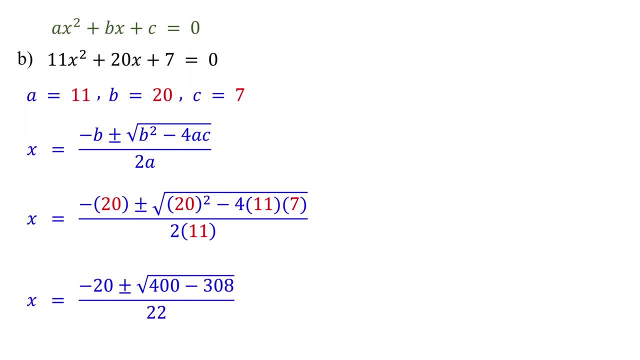 In the denominator 2 times 11 is 22.. 400 minus 308 is 92.. 92 is not a perfect square, but let's see if we can factor out a perfect square. to simplify, Let's do a prime factorization. 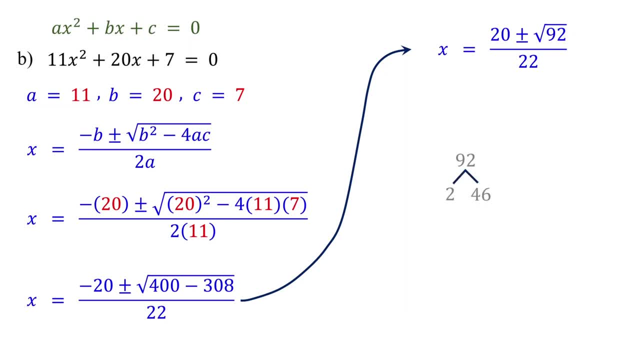 92 can be factored into 2 times 46. And 46 can be further factored into 2 times 46. And 46 can be further factored into 2 times 23,. right, Since 23 is a prime number, we cannot factor any further. 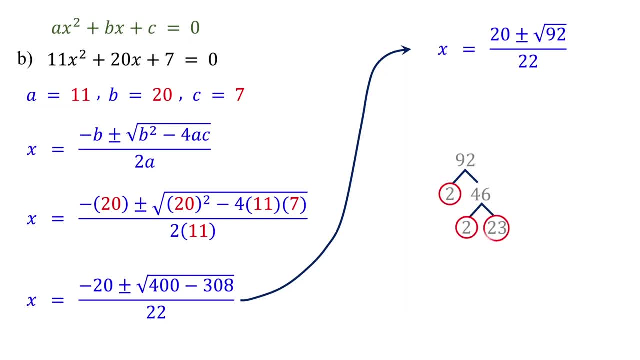 So 92 is the same as 2 times 2 times 23,, which equals 4 times 23.. This means 4 is the highest perfect square We can factor out from 92. Notice that these numbers have 2 as a common factor. 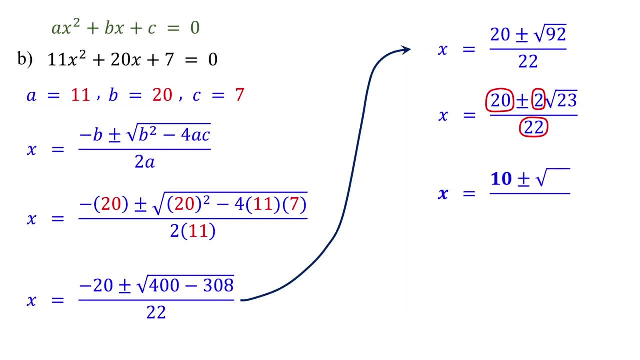 So we can simplify this by dividing each of them by 2, right, You can leave your solution as it is, Or you can also write it to show the two solutions separately. Both of them are acceptable ways of writing the solutions. Notice that both this example and the previous one have 2 real solutions. 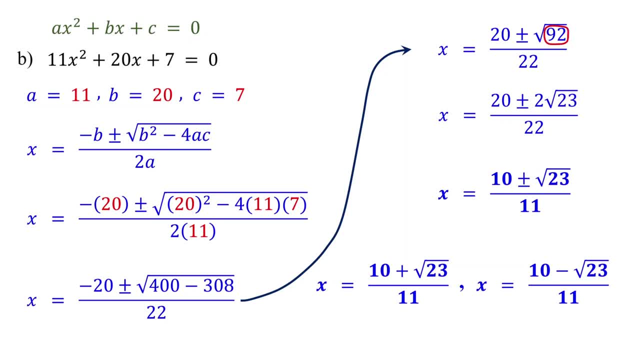 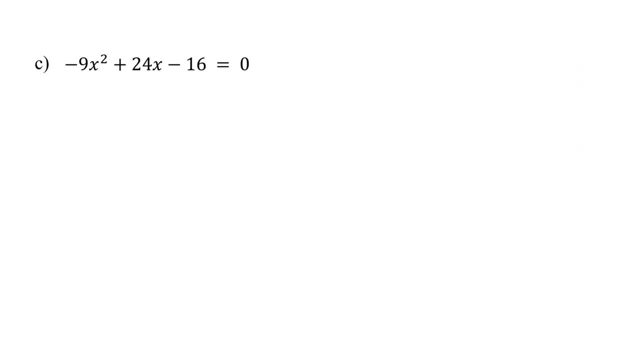 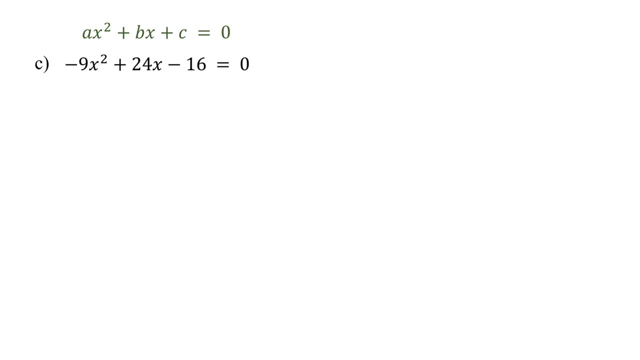 Since it is in standard form. first identify the values of the coefficients: A is negative 9,, B is 24, and C is negative 16.. Next write down the quadratic formula. Then substitute the values of the coefficients into the formula. 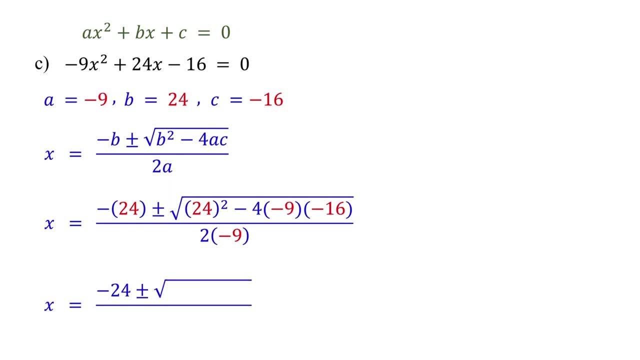 Now simplify this: Inside the square root, 24 squared is 576.. 4 times negative: 9. Is negative: 36.. And negative: 36 times negative 16. Is 576.. In the denominator: 2 times negative, 9 is negative 18.. 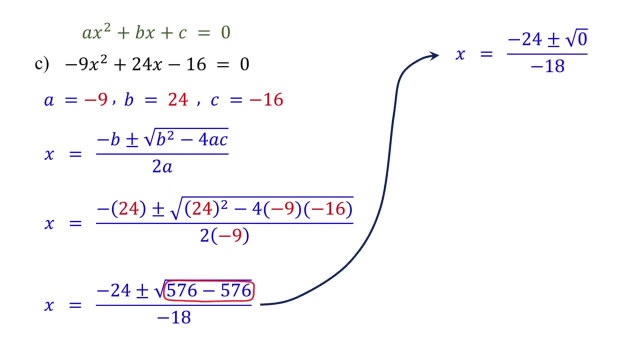 The difference inside the square root equals 0, right, The square root of 0 is 0.. Adding or subtracting 0 doesn't change anything, So we are left with negative 24 over negative 18.. If we divide both of them by negative 6,. 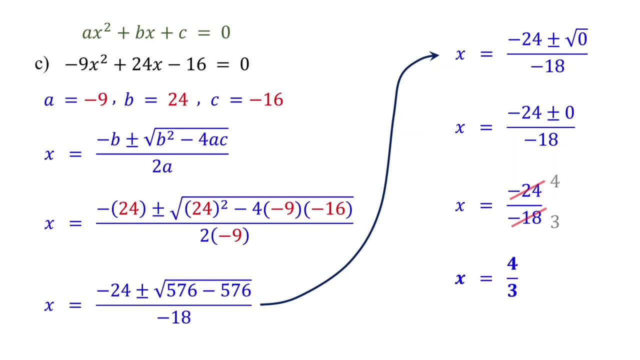 it simplifies everything. That's 4 times 4, right. Notice that this quadratic equation has only one real solution. This happens when the number inside the square root is equal to 0.. Finally, let's consider a case where a quadratic equation has no real solutions. 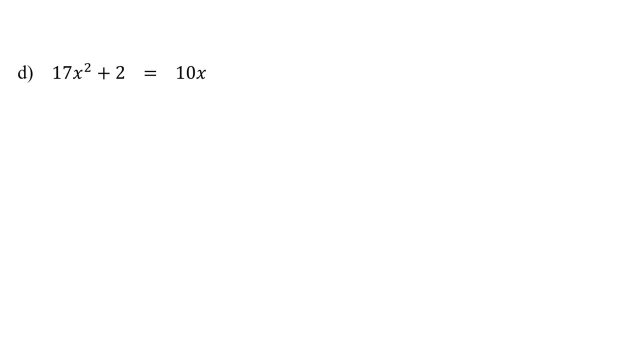 In the previous three examples, the quadratic equations were given in standard form. However, in this example, it is not To use the quadratic formula. the quadratic equation must be written in standard form. So our initial step here is to find the quadratic equation. 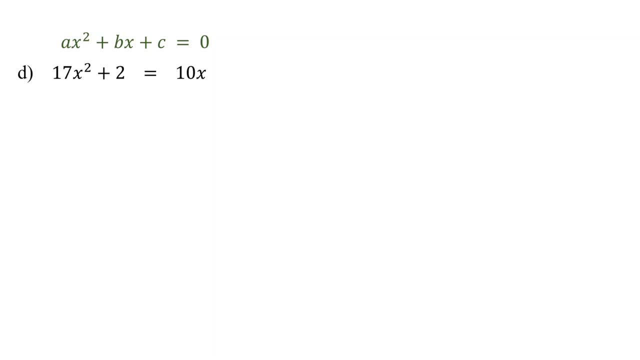 The first step here is to rewrite this equation in standard form. To do this, subtract 10x from both sides of the equation. Next identify the values of the coefficients: a is 17,, b is negative 10, and c is 2.. 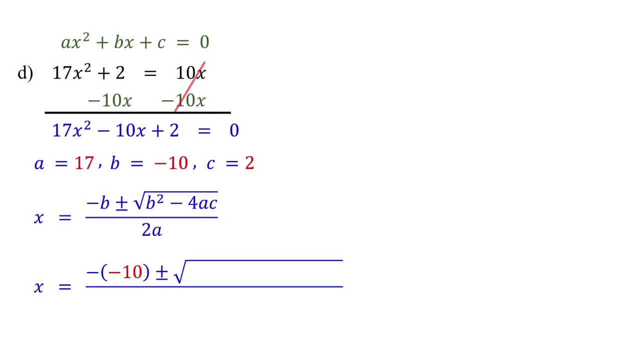 Then write down the quadratic formula and substitute the values of the coefficients into the formula. Now simplify this In the numerator: the negative of negative 10 is positive 10.. Negative 10 squared is 100.. 4 times 17 is 68, and 68 times 2 is 136.. 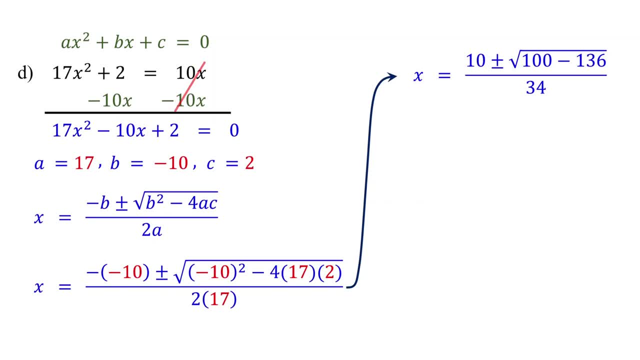 In the denominator 2 times 17 is 34.. 100 minus 136 is negative 36, right. Notice that the number inside the square root is negative. Now, if you are in Algebra 1, you are working within the root of the square root. 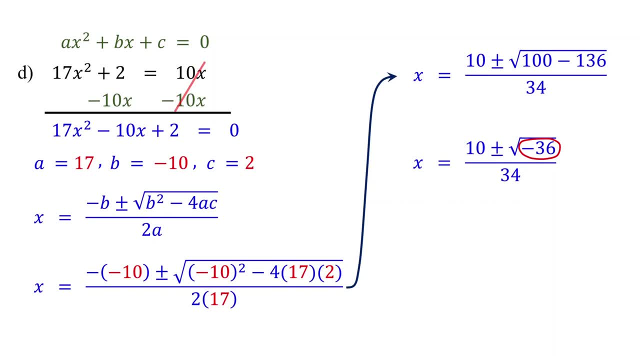 In the real number system, we cannot take the square root of a negative number right, So the answer to this problem is there are no real solutions. However, if you are in Algebra 2, this problem instead has two complex solutions. 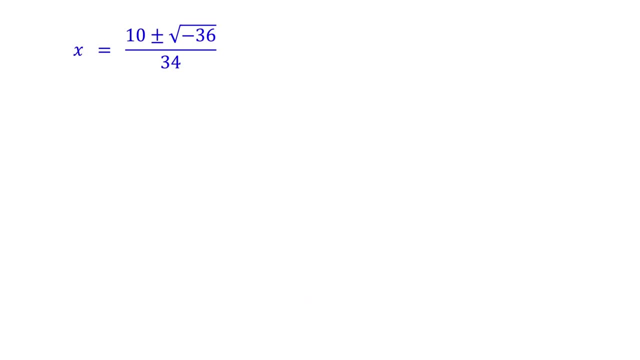 So we have a few more steps to do. Negative 36 is the same thing as 36 times negative 1, right, This equals the square root of 36 times the square root of negative 1.. The square root of 36 is 6.. 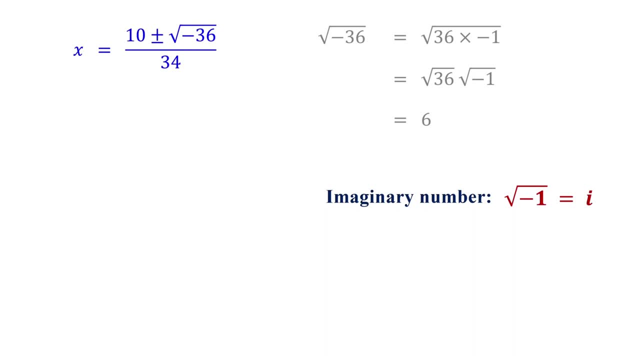 From the definition of imaginary numbers, the square root of negative 1 is denoted by i. So here we replace the square root of negative 1 with i. Therefore, the square root of negative 36 is 6i. Notice that 10,, 6, and 34 all have 2 as a common factor. 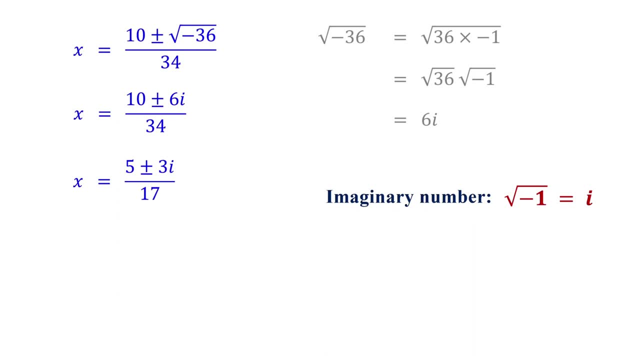 So we can simplify this by dividing each of these numbers by 2, right? Since this is a complex number, you need to rewrite it in the standard form of complex numbers, which represent it as a plus bi, where a and b are real numbers. 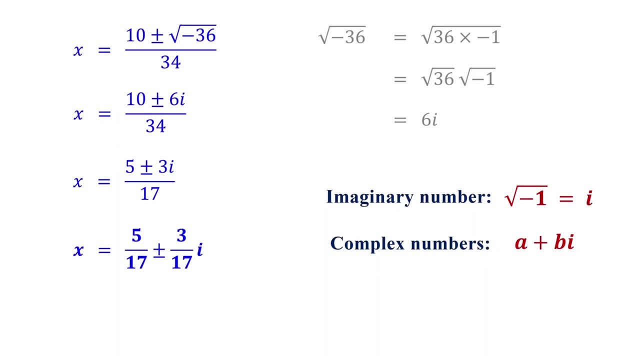 So we have 5 over 17 plus or minus 3 over 17i. You can either leave your solution as it is or write it to show the two solutions separately When solving the quadratic equations. you have observed that for the first two examples.